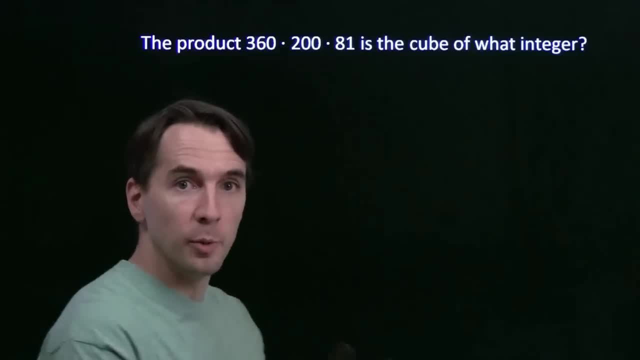 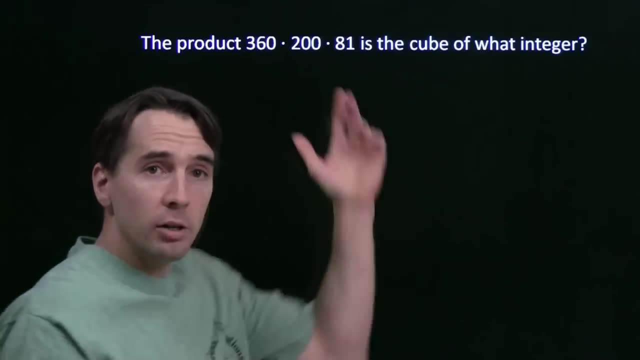 I think of the primes as building blocks of the integers. It's just one group of primes you can multiply together to get 360. That's the prime factorization of 360. Same thing for 200 and for 81. So I'm going to start this problem just by finding the prime factorizations. 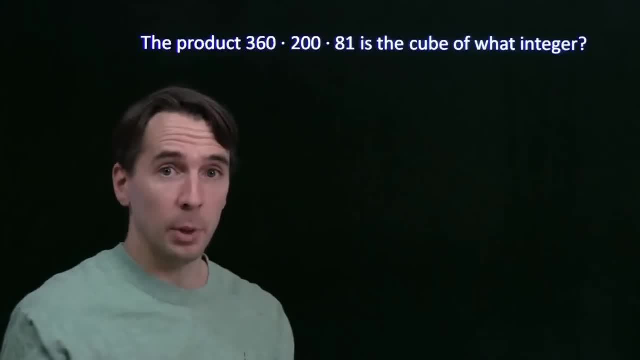 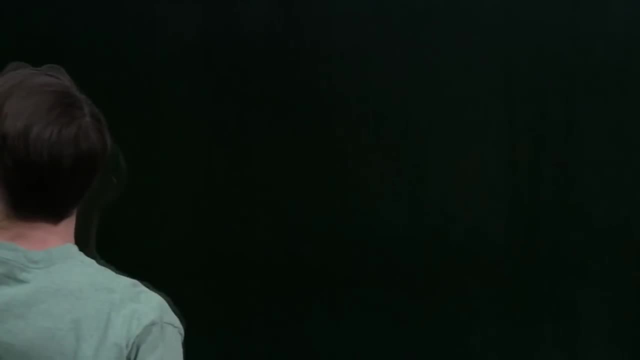 of these three numbers. Now I don't know for sure that getting the prime factorizations is going to help me solve the problem, But sitting here and staring at the problem isn't going to help either. So rather than sit and stare, I'm going to do something and hope it turns out to be something smart. 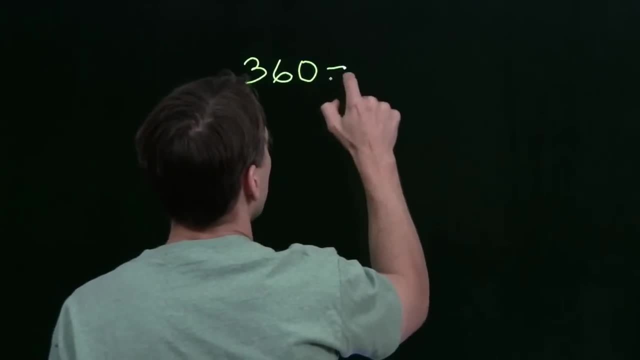 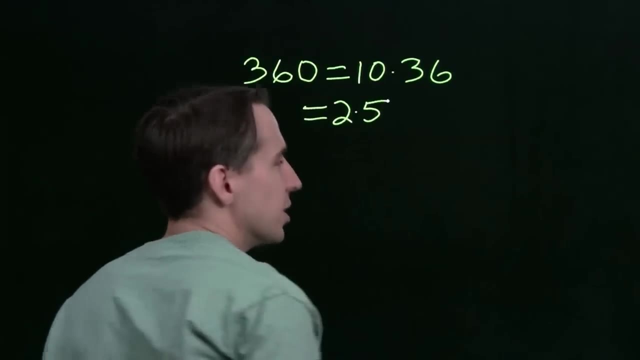 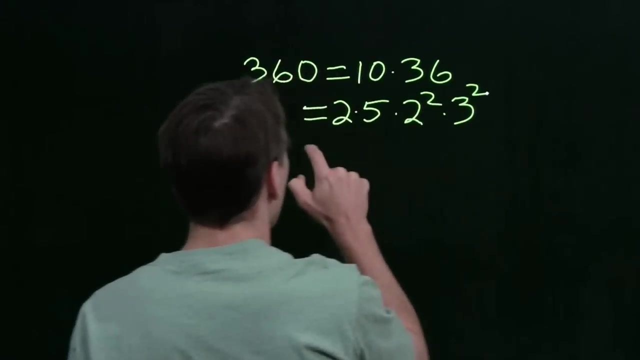 So we'll start with 360.. We're going to find the prime factorization of that. That's just 10 times 36.. Let's see: 10 is 2 times 5.. 36 is 4 times 9.. 4 is 2 squared. 9 is 3 squared. 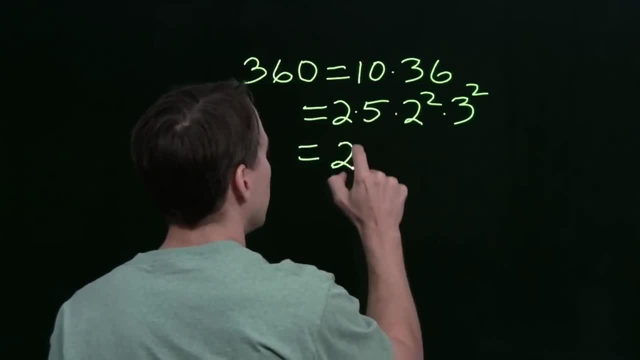 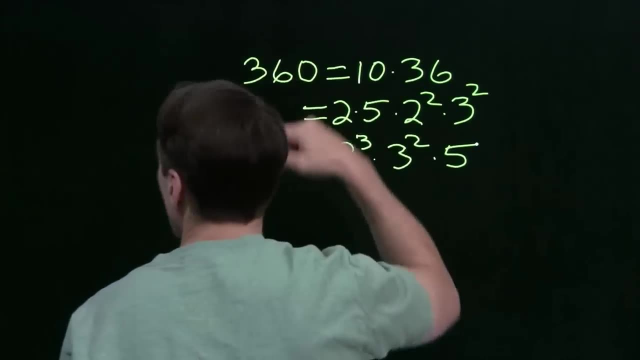 Now I can combine the two And the 2 squared. that gives me 2 cubed. I have the 3 squared and I have the 5.. So there's my prime factorization of 360.. We'll go ahead and write that down back here and 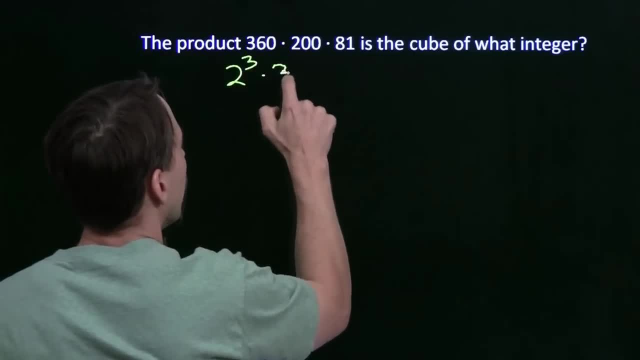 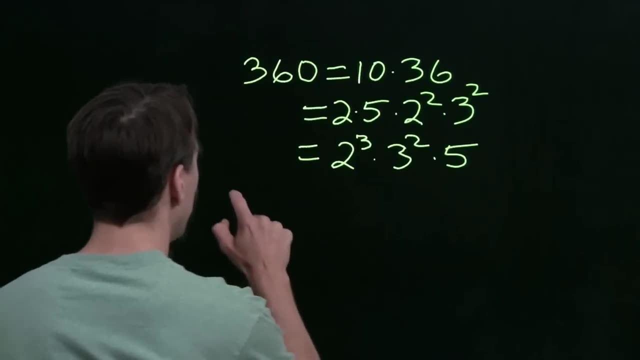 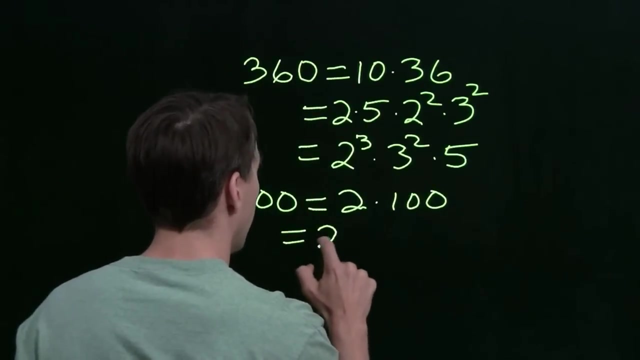 hope it proves to eventually be useful. This is 2 cubed times 3 squared times 5.. All right, 200.. Let's do 200, next 200.. Well, 200 is just 2 times 100.. And 100, well, that's 10 squared. So that's 2 squared times 5 squared, 2 squared times. 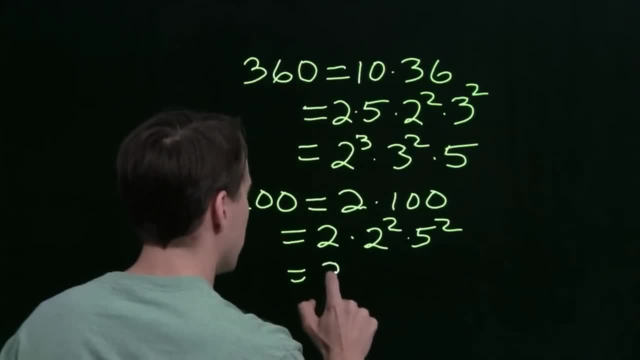 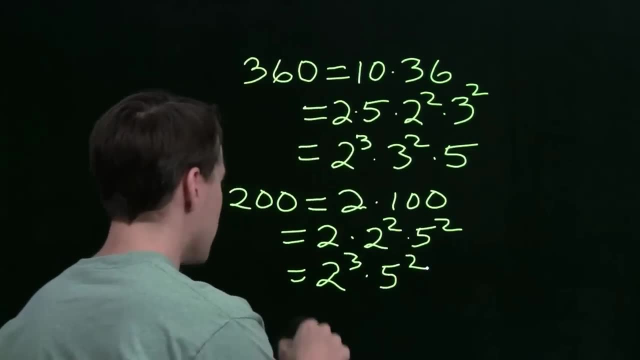 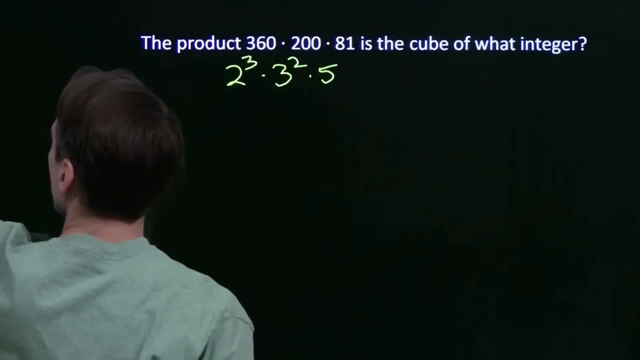 5 squared And that gives me a prime factorization of 2 cubed times 5 squared. I'm going to check that real quick. I like to check my intermediate steps just to make sure I don't mess up. 2 cubed is 8.. 5 squared is 25.. 8 times 25, that's 200.. We have the right prime factorization. 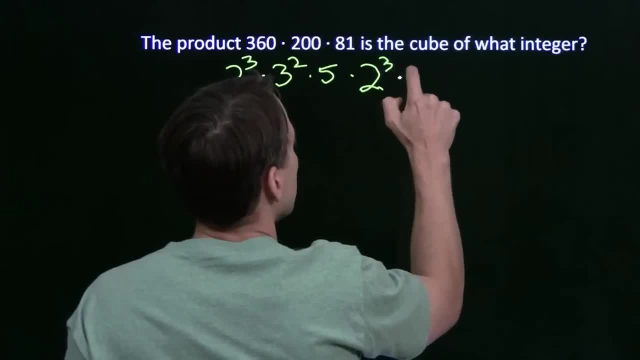 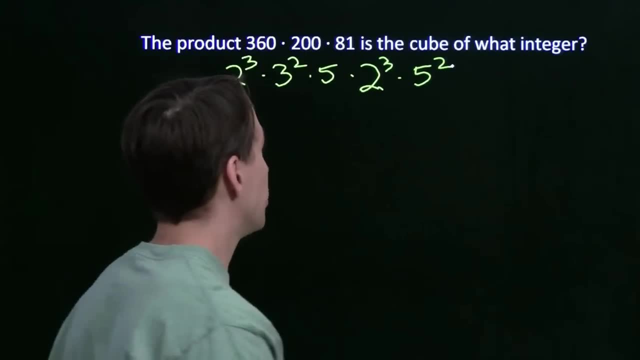 there. So this is just 2 cubed times 5 squared. All right, All right, All right, And 81.. 81 is just 9 times 9.. 9 is 3 squared, 3 squared times 3 squared. That is 3 to the. 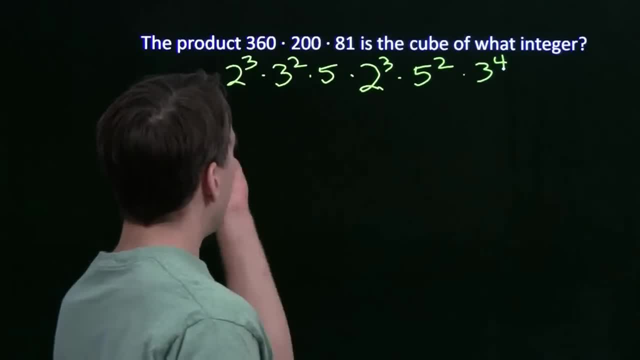 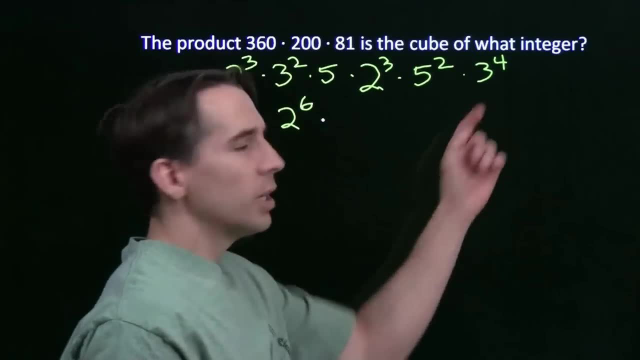 fourth. All right, Let's see. So now I can combine a bunch of these. I can combine 2 cubed and 2 cubed. That gives me 2 to the sixth, 3 squared and 3 to the fourth. That gives me 3 to the. 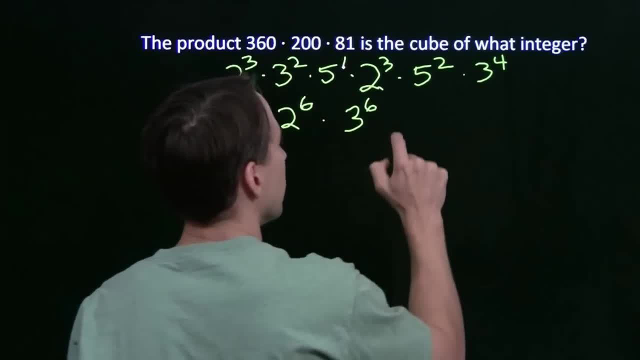 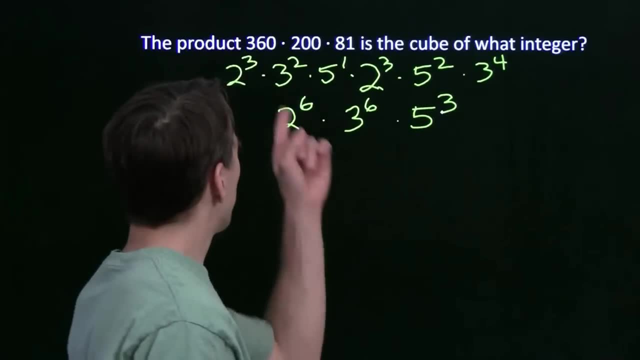 sixth, 5 and 5 squared, That 5,, of course, is 5 to the first, So we have 5 cubed. Well, that looks a little simpler than this. Maybe. I mean if all the exponents were 3,. 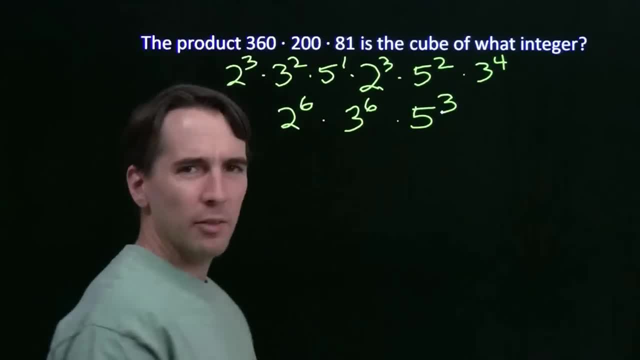 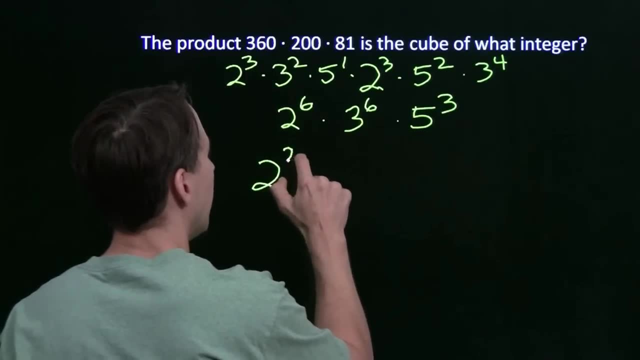 we'd feel really close because we're looking for the cube of an integer. We have those 6's sitting there. I can write: 6 is 2 times 3.. Let's check that out. Write: each of these exponents of 6 is 2 times 3, because in the end we want a cube, We want a cube of an. 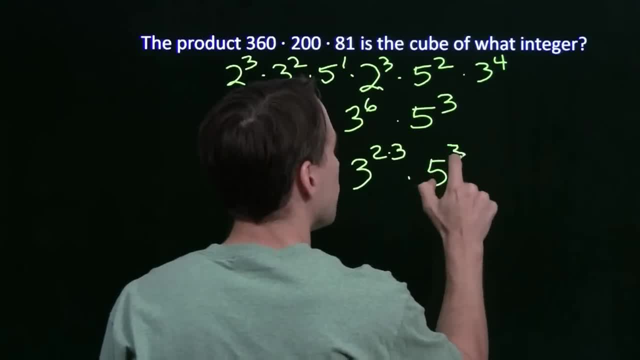 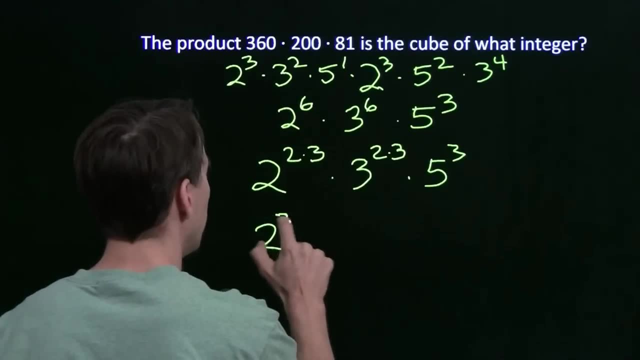 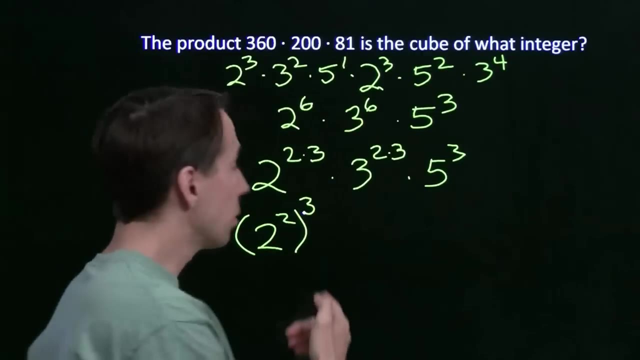 integer. And now we can use one of our exponent rules. We can use one of our exponent rules. We can write this as the cube of an integer, We can write this as the cube of 2 squared, And it's just our power of a power, rule 2 squared raised to the third. We just multiply the. 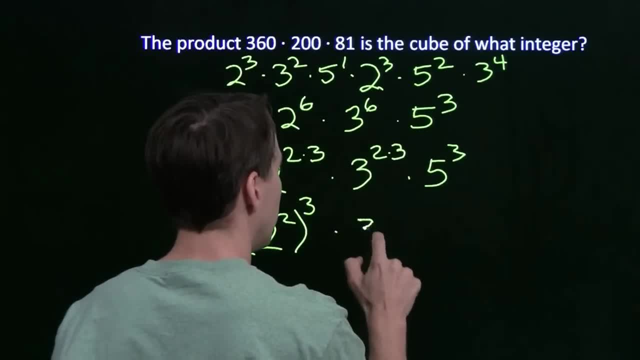 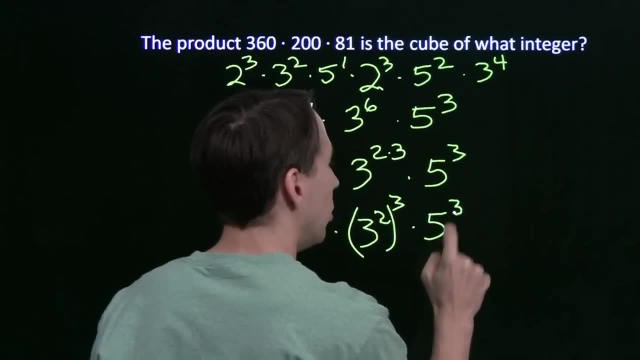 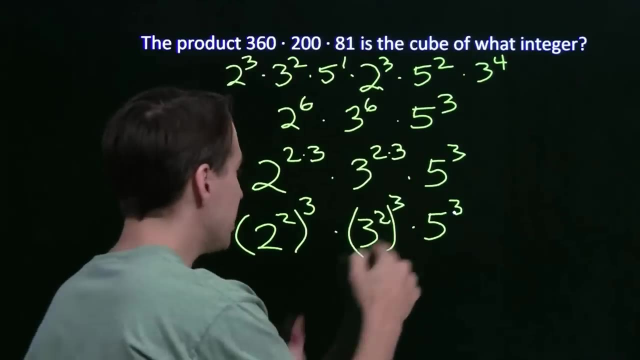 exponents 2 times 3.. Go in the other direction. here We do the same thing with the 3. And now we have a product of cubes. Same exponent. We know how to multiply powers that have the same exponent. We have another exponent rule. 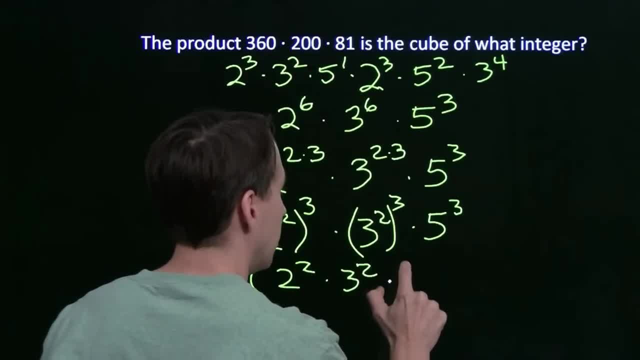 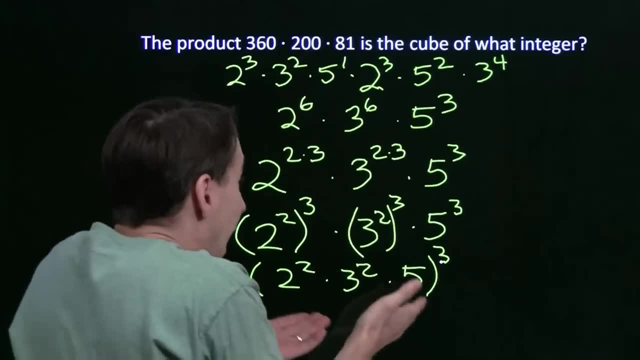 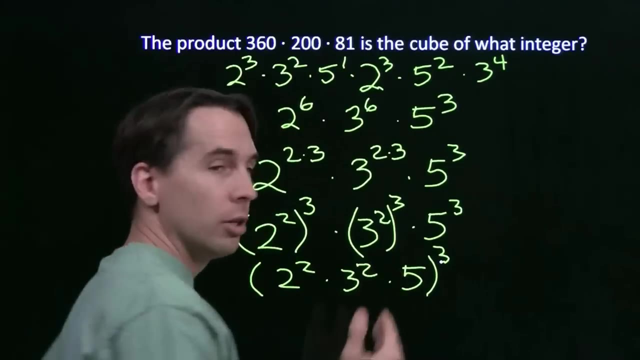 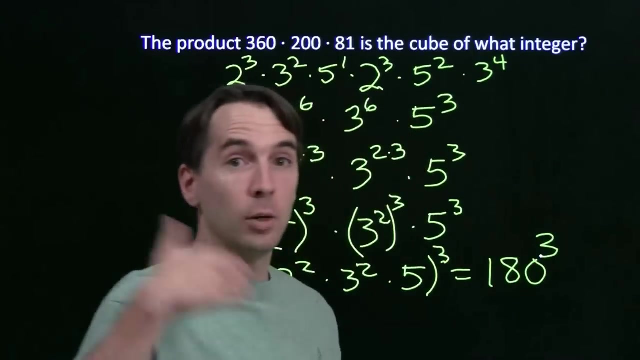 for that We have a product of cubes. Well, that's just the cube of the product of the numbers. We have the cube of an integer. All we have to do is compute this integer: 2 squared is 4.. 4 times 5.. That's 20.. 3 squared is 9.. 9 times 20.. That's 180.. 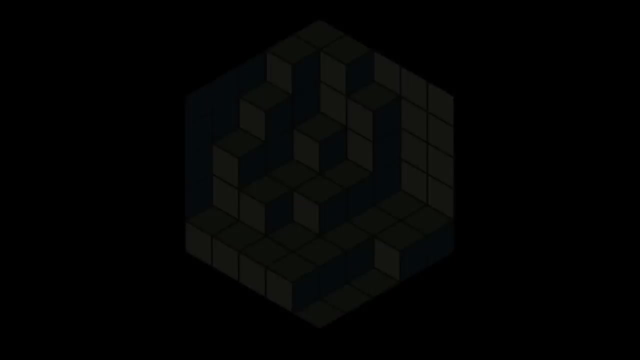 And we are done, And we are done, And we are done.